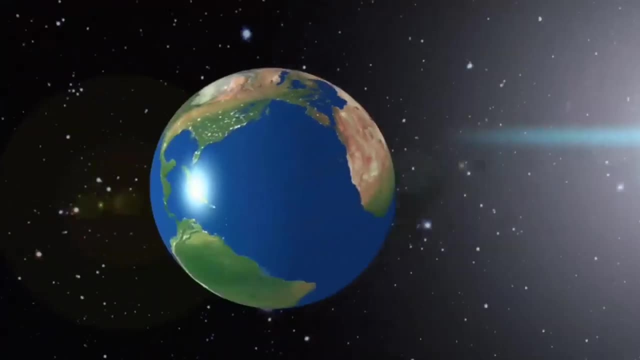 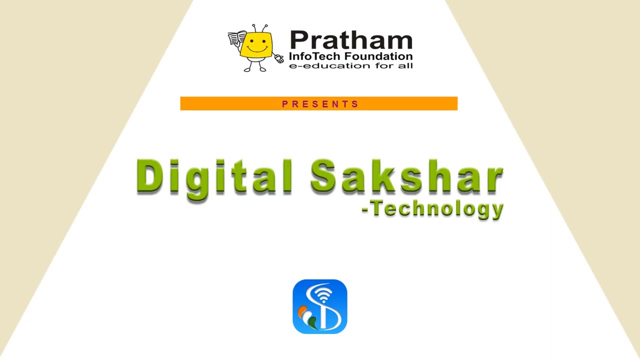 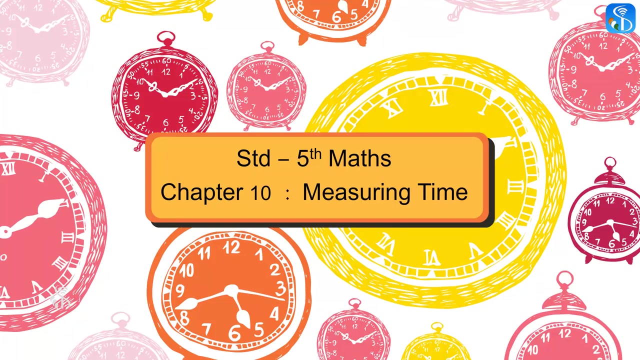 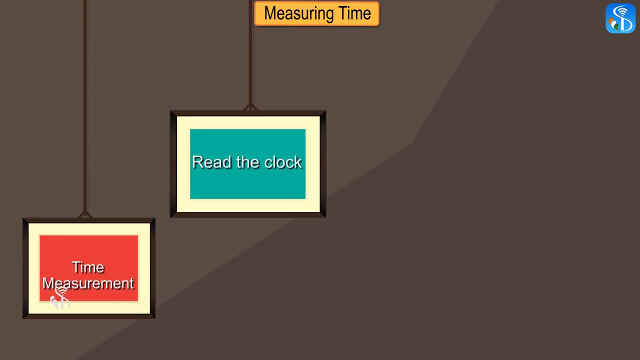 Standard 5th. Subject: Math. Chapter 10: Measuring Time- Children. we have studied time measurement in 3rd and 4th standard. We have learnt to read the clock about the days of the week, months of the year and so on. 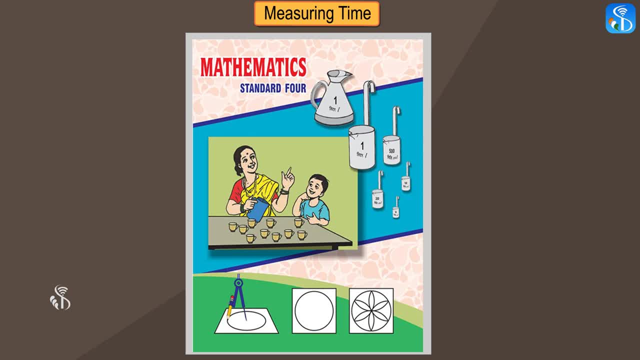 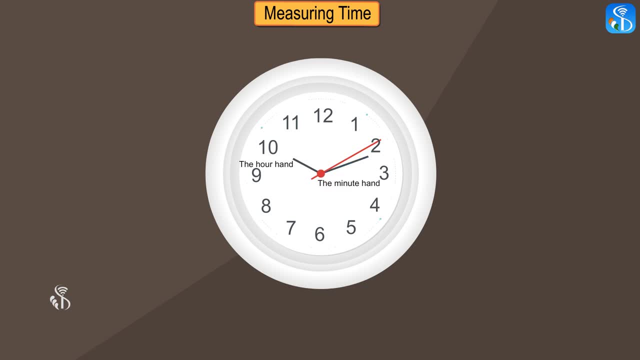 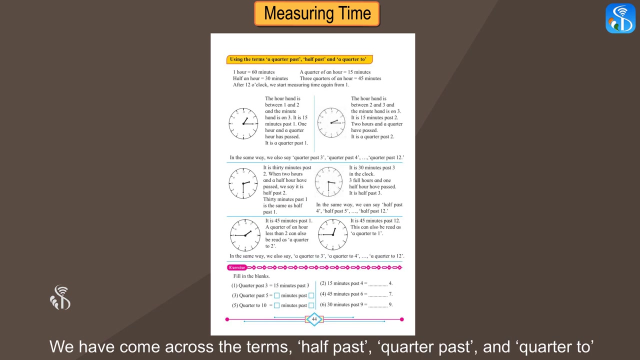 Last year. we have learnt about the two hands of the clock: the hour hand and the minute hand. You know that 1 minute is equal to 60 seconds and 60 minutes is equal to 1 hour. We have come across the terms half past, quarter past and quarter to, and know their meanings. 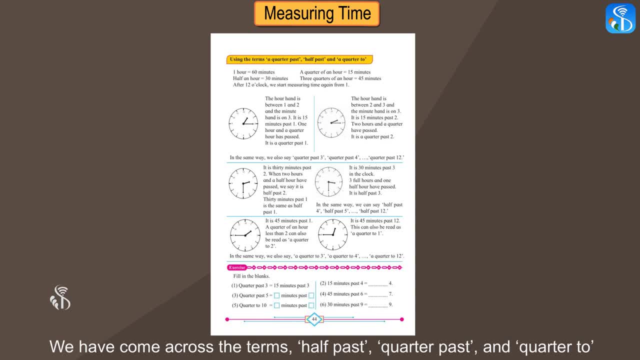 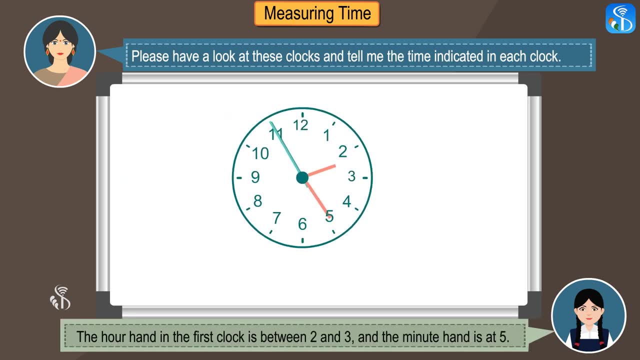 Today we are going to revise these concepts with the help of Children. please have a look at these clocks and tell me the time indicated in each clock. Ma'am. the hour hand in the first clock is between 2 and 3 and the minute hand is at 5.. 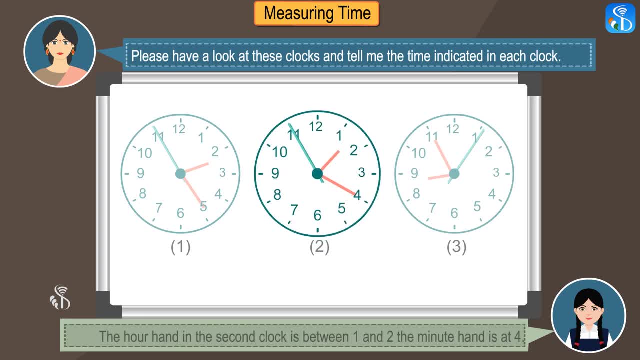 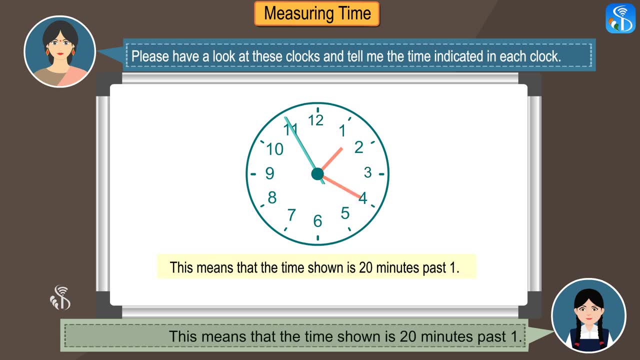 Therefore, the time shown in this clock is 25 minutes past 2.. Ma'am, we can see that the hour hand in the second clock is between 1 and 2.. The minute hand is at 4. This means that the time shown is 20 minutes past 1.. 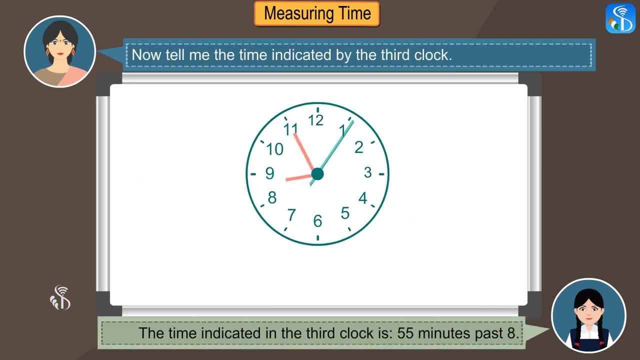 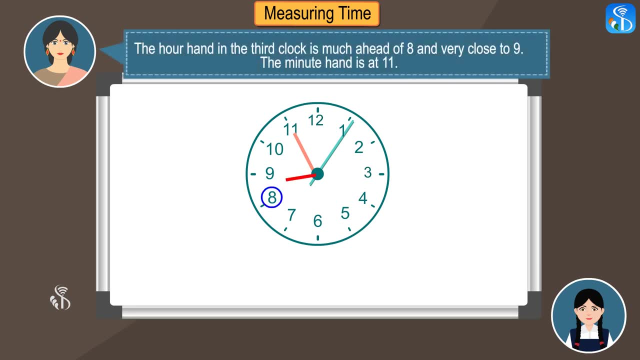 That's right. Now tell me the time indicated by the third clock. The time indicated in the third clock is 55 minutes past 8.. Very good, Look here. The hour hand in the third clock is much ahead of 8 and very close to 9.. 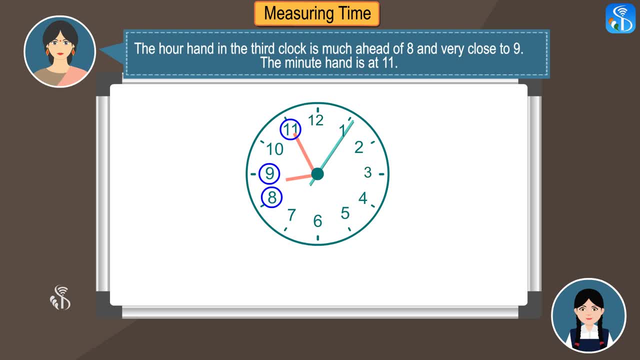 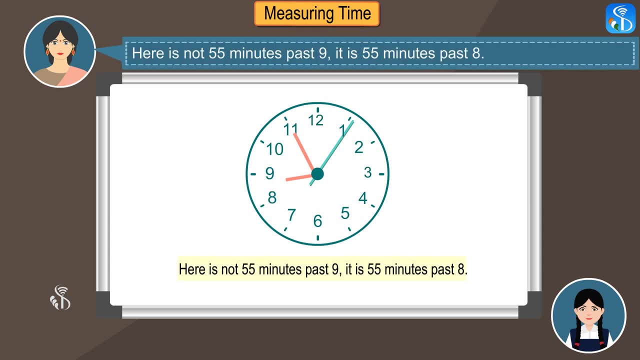 The minute hand is at 11.. Many students get confused by this position of the hour hand. They say the time is 55 minutes past 9.. But in fact the time indicated here is not 55 minutes past 9.. It is 55 minutes past 8.. Okay. 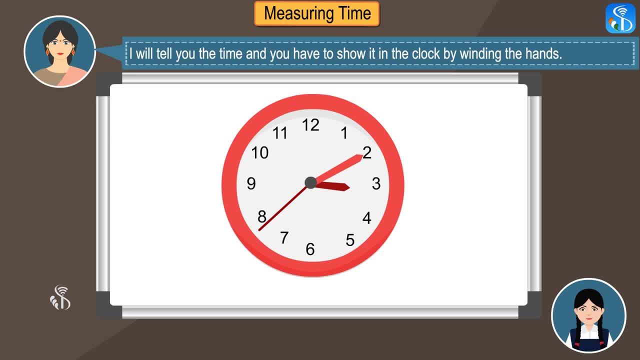 Now I will tell you the time and you have to show it in the clock. You have to show it by winding the hands. It is quarter past 3 now. Quarter past 3 means 15 minutes past 3.. So the hour hand will be a little ahead of 3 and the minute hand will be exactly at 3..